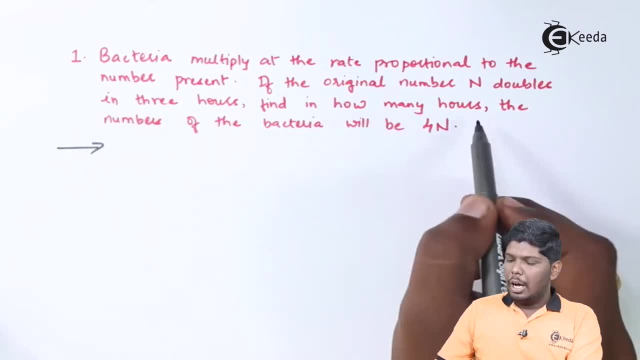 n doubles in 3 hours, find in how many hours the number of the bacteria will be 4n. They have told you that the increase in number of bacteria is proportional to the original number. It is but obvious that if I say that the number of bacteria is proportional to, 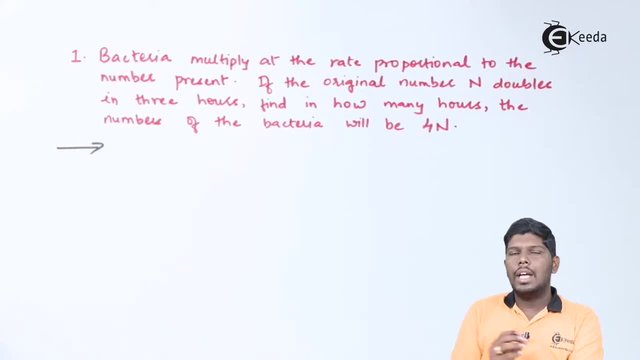 the number of bacteria. then I am saying that at starting there are 100 bacteria and in the second we have 10,000 bacteria. The rate of growth will be in the second case only. As the number of bacteria is more there, the rate of growth will be also more, So they. 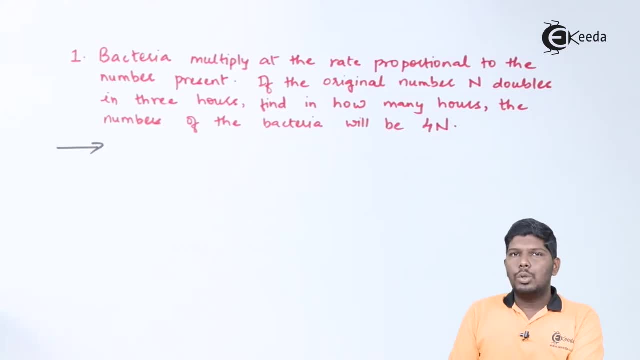 have given you the same information. Now, two things that we are supposed to assume is that the number of bacteria at any time t. So let us assume that there are X number of bacteria at any time t. Now let us use this first equation in order to get the differential equation: Bacteria. 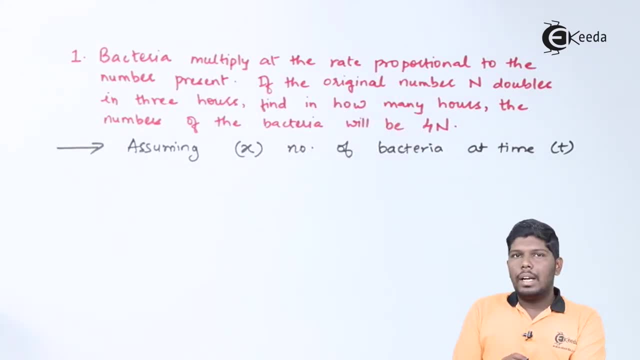 multiply at the rate of proportional. So change in number of bacteria with respect to time, Change in number of bacteria that will be dx With respect to time that will be dt, Is directly proportional to the number of bacteria present, Number of bacteria we have assumed. 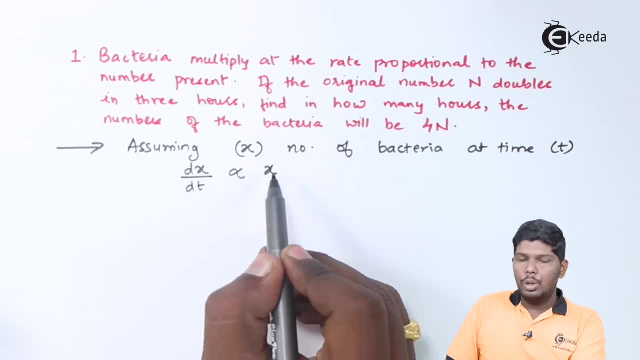 that it is X. So dx by dt is directly proportional to X. Now, removing this proportionality sign, we should give the constant of proportionality. Therefore, let us assume that constant is k and dx by dt will be equal to kx. Now remember: whenever there is growth, we will write plus. 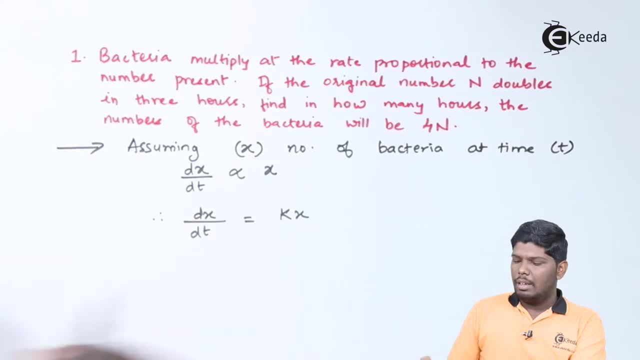 k and whenever there is decay or less, we will write minus k. After that we can separate the variables, solve it using variable separable form and get the general equation On separating variables. we have: dx by x is equal to k, dt, And let us integrate on both. 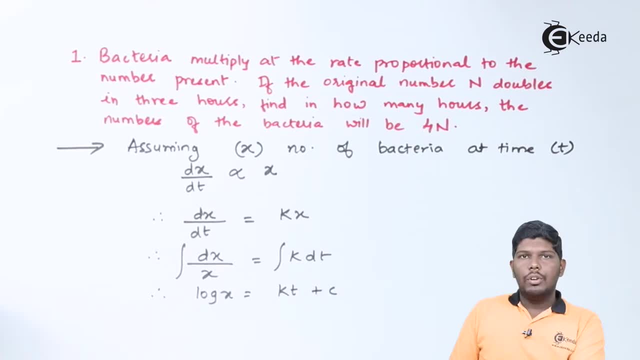 sides. So we will get log: x is equal to kt plus c. So this is our first equation. Now let us use these conditions in order to get the values of constant and k, For that first condition is given as if the original number n doubles in 3 hours, So the original number 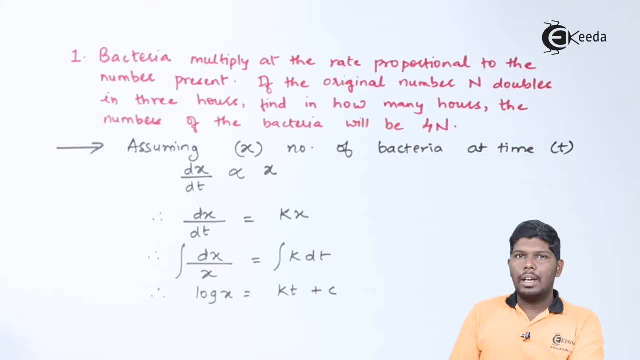 was n. Original number means it is a starting number of bacteria And for that we can take the value of time as 0. As from that time we are going to start the process. So when time is 0, number of bacteria, that is, x, will be equal. 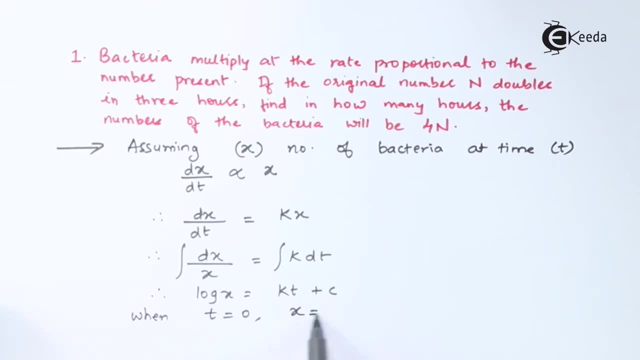 to n. Let us use this value in the above equation and get the value of first constant, So x will become n. That will give you log n. Value of t is 0. So k into 0 will be 0, only plus. 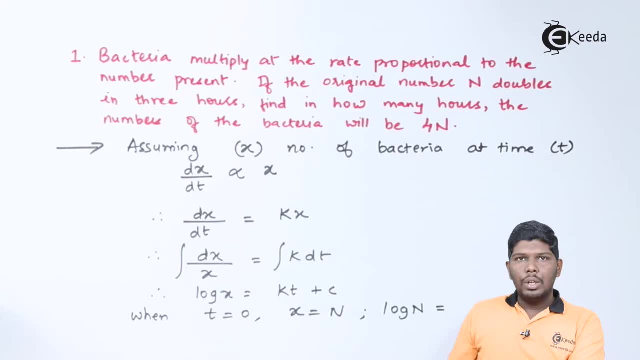 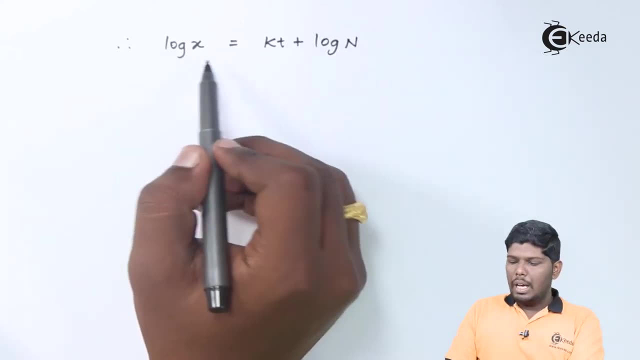 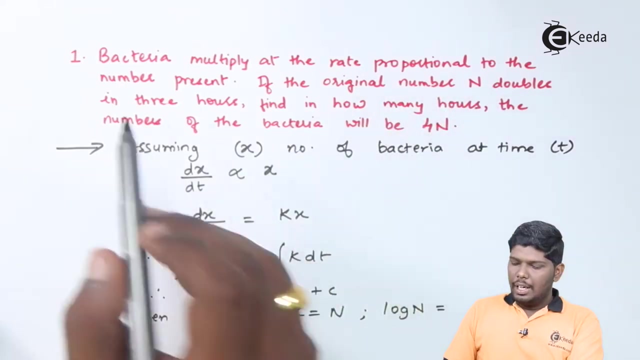 c. So k into n is equal to log n. Now substitute the value of c in the above equation. Therefore we have: log x is equal to kt plus log n. The second information says the original number n doubles in 3 hours. The initial time was 0. At that time number of bacteria was 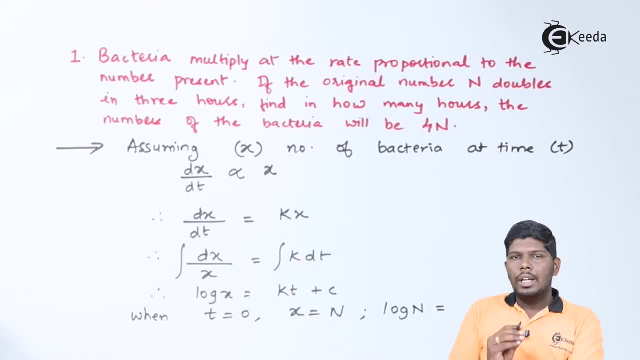 n After 3 hours. when t is 3 hours, the number of bacteria is doubled. Previous it was n, So now it will be 2n. If I say the previous it was 100, now the double will be 200.. Similarly, 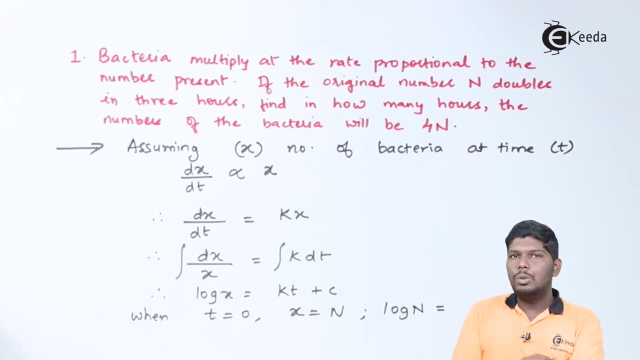 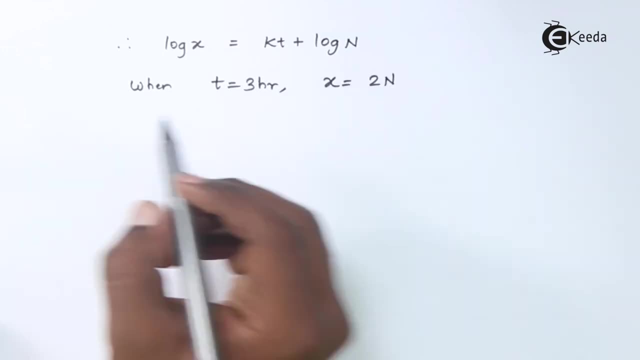 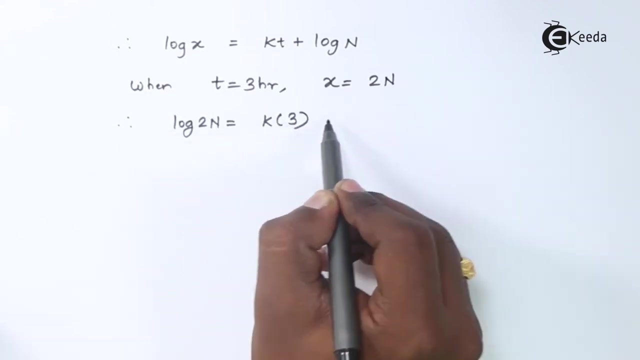 the previous it was n. its double will be 2n. Let us use this condition to get the value of second constant, that is, k. When time is 3 hours, number of bacteria x will be equal to 2n. By solving this equation we will find: 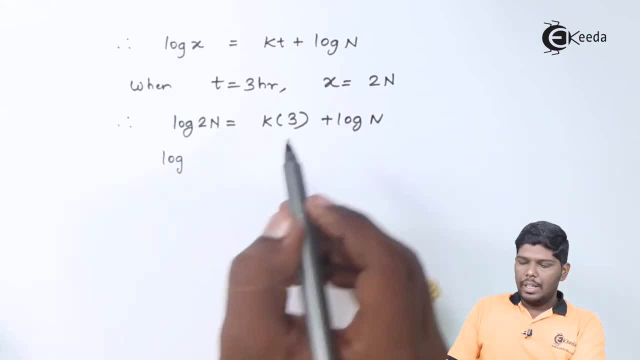 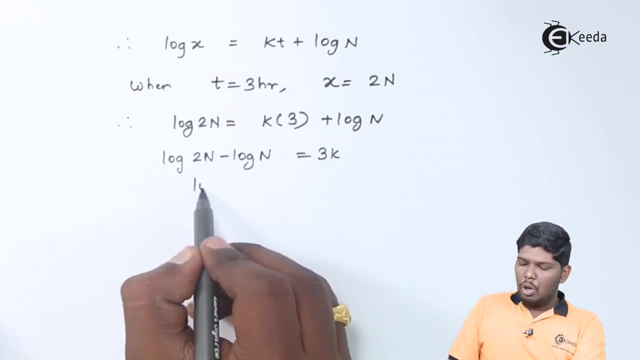 the value of k Taking n. on the left hand side we have log2n. minus logn is equal to 3k. Log a minus log b will give you log a by b, where n will be cancelled, 3 will be divided and the value of k will be 1 by 3 log2.. 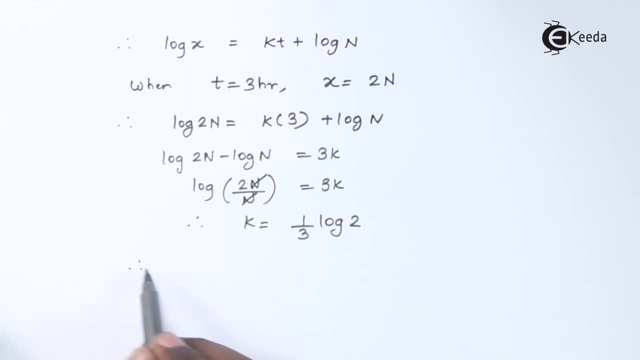 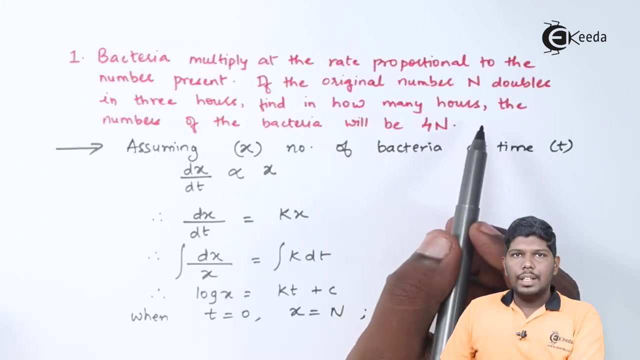 Again, we will substitute the value of k in the above equation. This will give you: logx is equal to the value of k, is 1 by 3, log2 into t, as it is plus logn. Now let us use the last condition to find the answer.